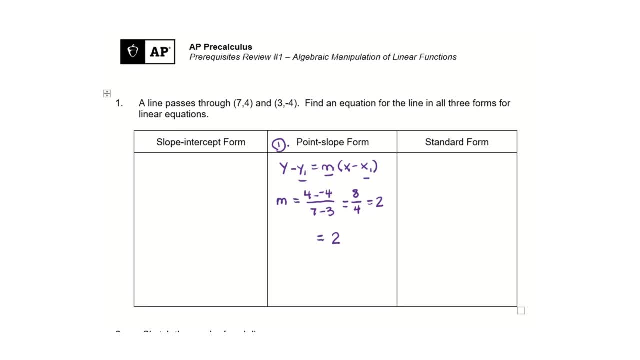 one. you use. both of them will give you an equation for the exact same line. I'm going to use the coordinates of the first point, so it's y minus x minus x, And I'm going to use the coordinates of the first point, which is 4.. And then, over here on the right side of the equation, 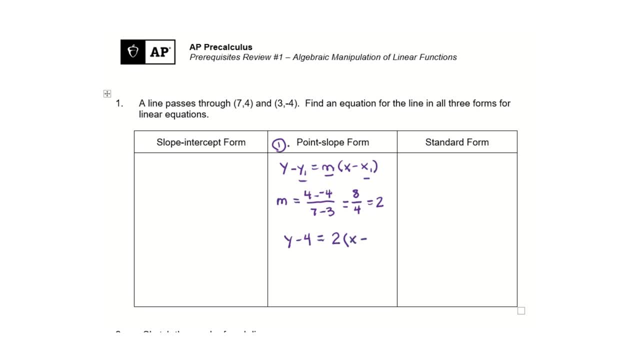 in the parentheses- it's going to be x minus the x coordinate of that point, which is 7.. So y minus 4 equals 2 times the quantity x minus 7.. Now that I've got an equation in point-slope form, 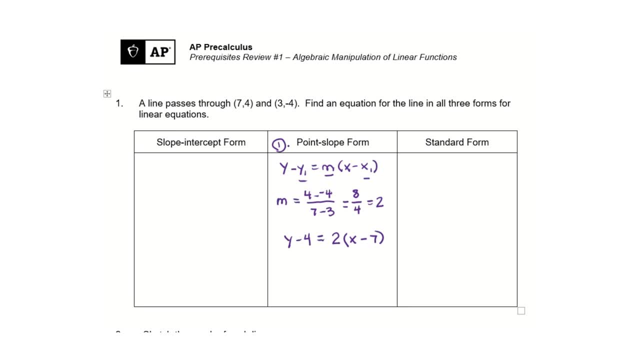 I can just rearrange that equation in order to find the equation in slope-intercept form. Slope-intercept form is the equation in point-slope form and slope-intercept form is the equation in point-slope form. Slope-intercept form is: y equals mx plus b. This is one that you probably see very frequently. 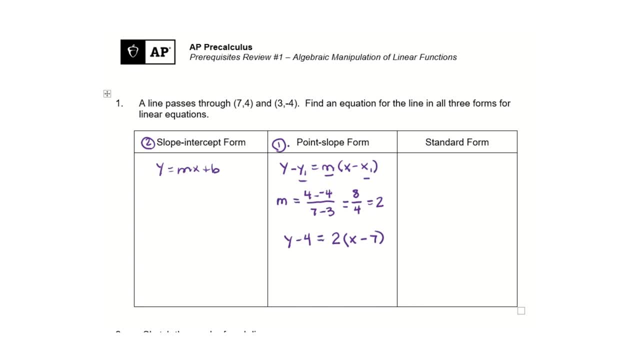 right, And you have seen it a lot since algebra 1.. So we already know what we're replacing the m with, That's a 2. But it would be really helpful to be able to figure out what we're replacing the b with. So we're going to take the equation that we already found in point-slope form, which is y. 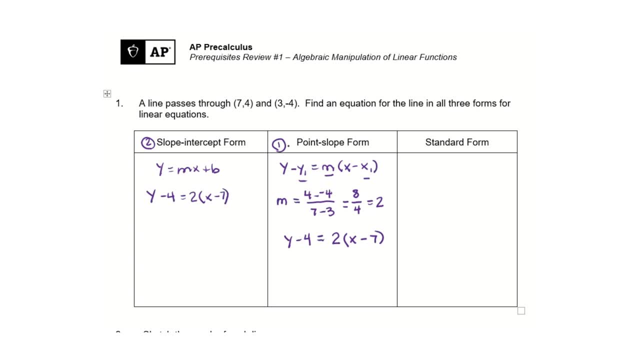 minus 4 equals 2 times x minus 7.. And we're going to simplify the equation, So we're going to start reading multiplication: 2 times x is 2x, and 2 times that negative 7 is negative 14.. So once. 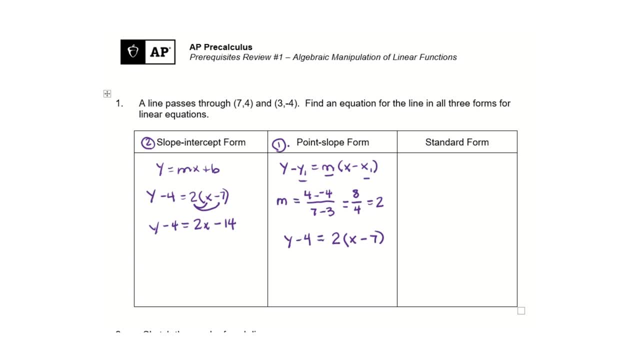 we've distributed, we have: y minus 4 equals 2x minus 14.. If we go back to slope-intercept form, y equals mx plus b. y is all alone, And so we're going to need to make sure that we get y all by. 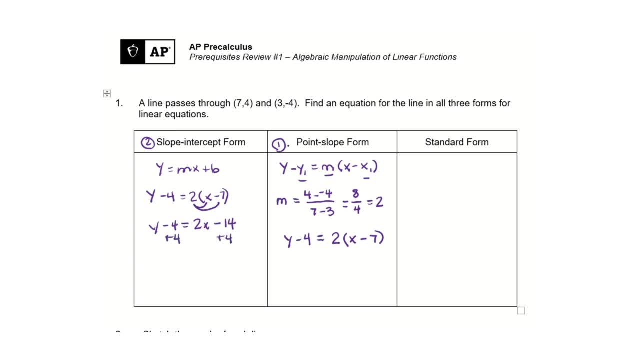 itself in this equation. We would do that by adding 4 to each side of the equation And the result will be y equals 2x minus 10.. Slope-intercept form is y equals 2x minus 10.. Next we can go on to finding. 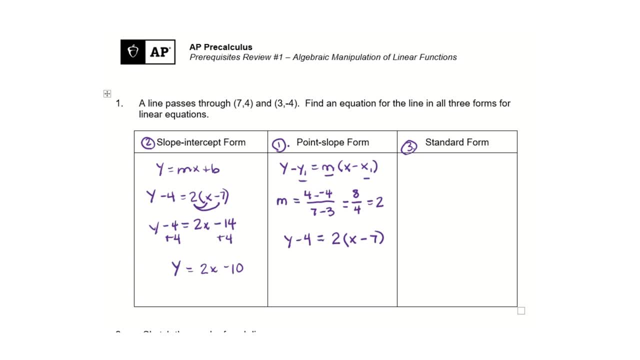 the standard form equation for this line. The standard form equation looks like this: ax plus by equals c. So we're going to need to take our slope-intercept form, which was y equals 2x minus 10, and get x and y on the same side of the equation. 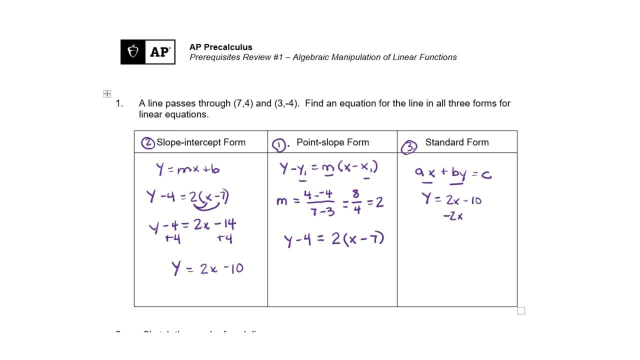 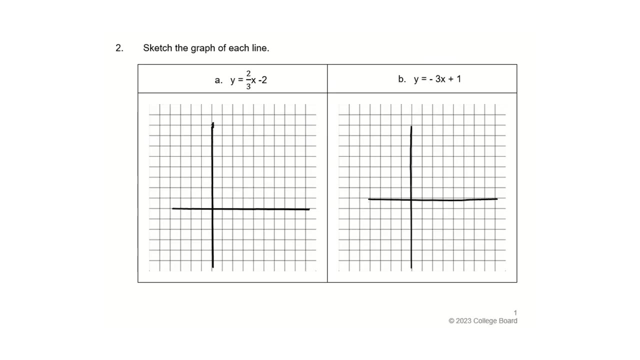 So we'll do that by adding negative 2x on each side of the equation, which will give us negative 2x plus y equals negative 10. And that's our standard form. equation In number 2, we're being asked to sketch: 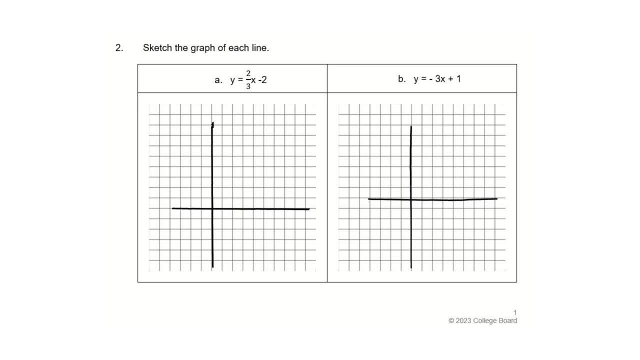 the graph of each line. Part a is y equals 2 thirds x minus 2, and part b is y equals negative 3x plus 1.. These equations are both in slope-intercept form, So to graph an equation in slope-intercept form. 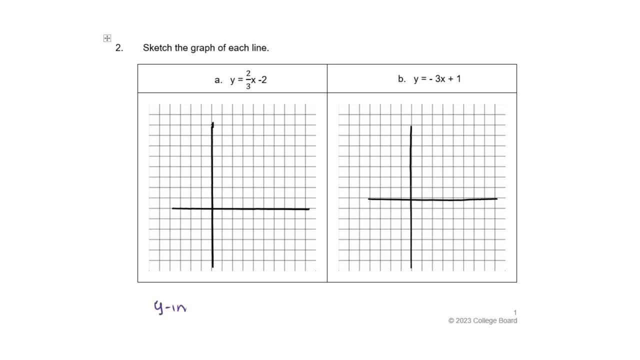 we always start with the y-intercept and then we navigate using the slope to find additional points. So in part a the y-intercept is negative 2.. So we're going to start at negative 2 on the y-axis and then we're going to use the slope. 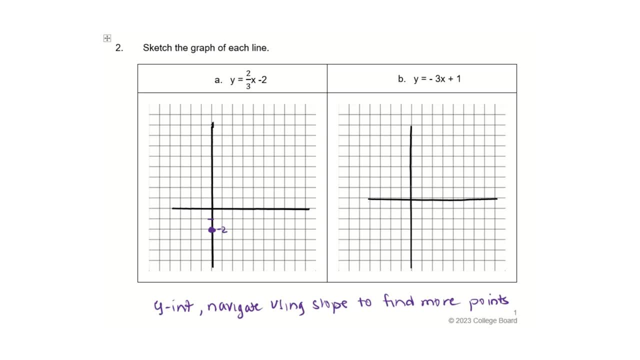 of two-thirds to find additional points. That's a positive two-thirds. so our rise is going to be positive 2, and our run is going to be positive 3.. So up 2 and to the right 3,, and that finds me. 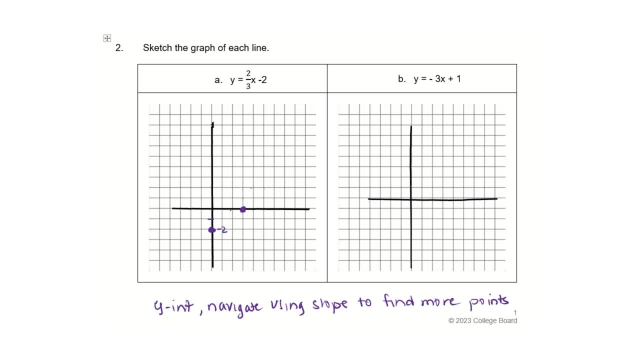 another point: Up 2 and to the right 3, and that finds me another point: Up 2 and to the right 3,, and that finds me another point. I could also reverse those directions. so I'm going back to the y-intercept of negative 2, and I'm going down 2, and to the left 3, because negative 2 and 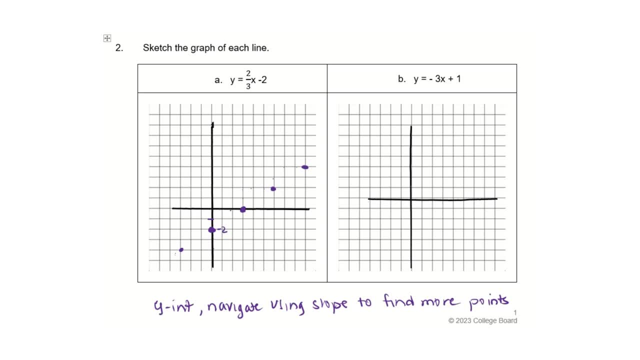 negative 3 would be a positive. When you divide two negative numbers you get a positive right. So here's my line, Very straightforward and simple. to graph that slope-intercept equation In part b, y equals negative 3x plus 1.. Again, we're going to start at the y-intercept, which is: 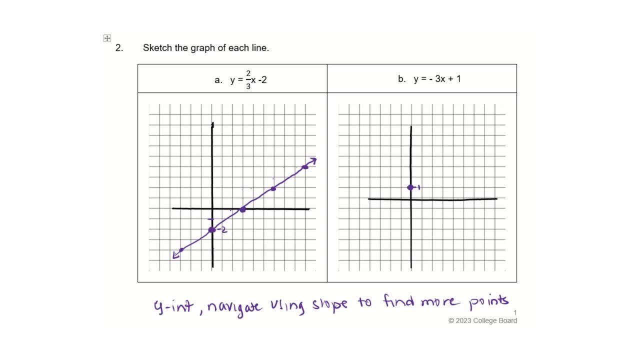 positive 1, and then we're going to use the slope of negative 3 to find additional points. Keep in mind: you need to think of that negative 3 as a fraction and that would be negative 3 over 1.. So that means we go down 3 and to the right 1, because when we make negative 3 a fraction, 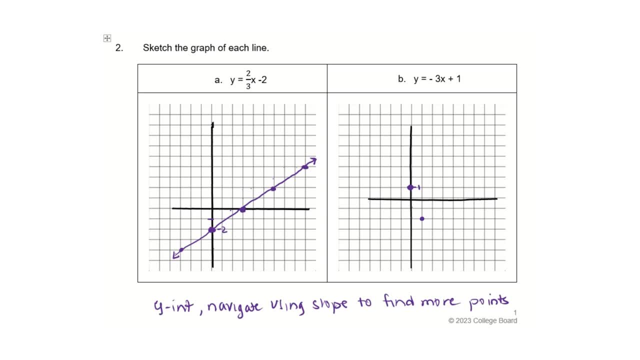 it's negative 3 over positive 1.. So negative 3, down 3 and to the right 1.. Or we start back at that y-intercept and we go up 3 and to the left, 1.. So when we mix a positive direction and a negative direction, we get a. 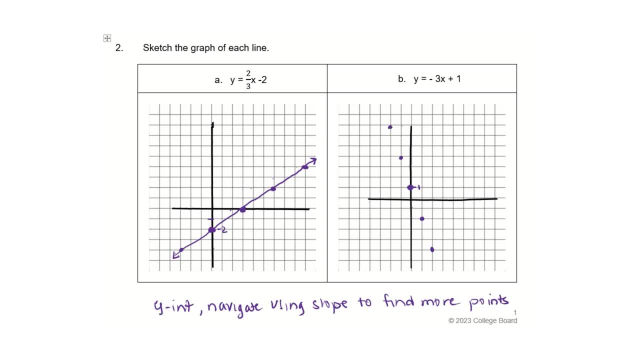 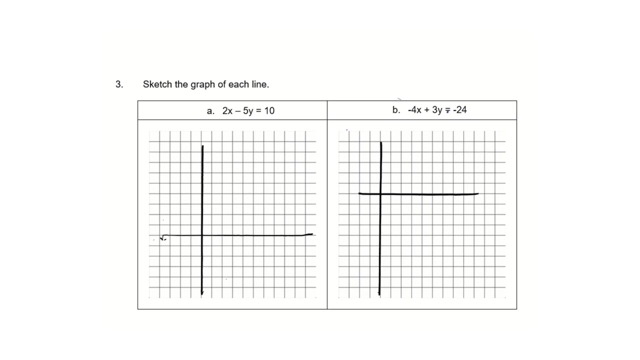 negative slope. So up 3 and to the left: 1. Negative slopes decrease from left to right. Positive slopes, like part a increase from the left to the right. Oh, that line was rough, but you get the idea. To sketch the graph of each line given to us in example three, we need to take a different. 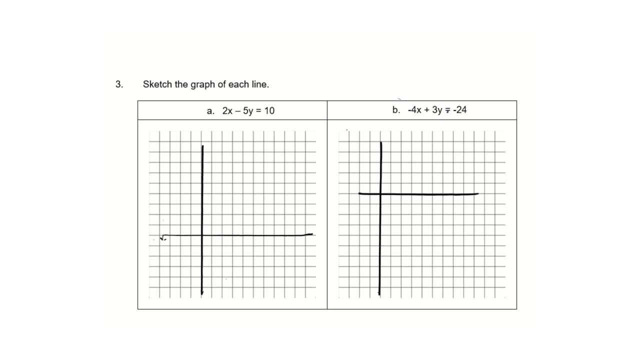 approach because these are not in slope-intercept form. Part a has the equation: 2x minus 5y equals 10, and part b has the equation negative 4x plus 3y equals negative 24.. These equations are in: 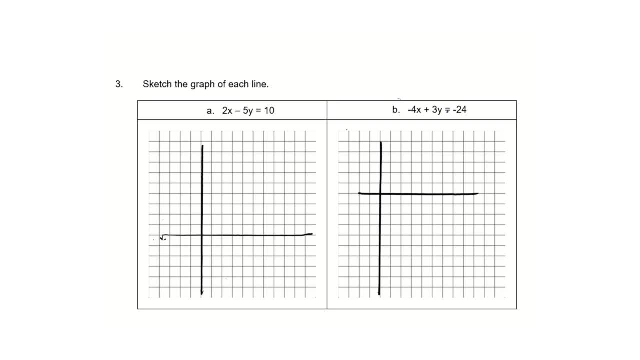 standard form. So when we have an equation that has a slope-intercept form, we need to take a different approach. So when we have an equation in standard form, we typically would start out by finding the x-intercept and finding the y-intercept, graphing those points and then drawing the line. 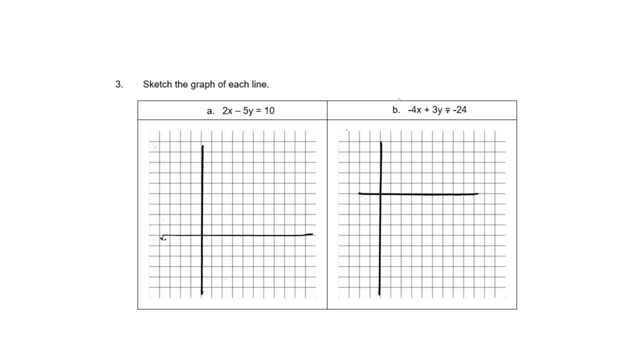 from there. If you think about it, since the x-intercept is the value of x when y equals 0, we can find the x-intercept quickly by thinking about the equation: 2x equals 10.. The x-intercept in this case is going to be 5. To find the y-intercept? that's the point. 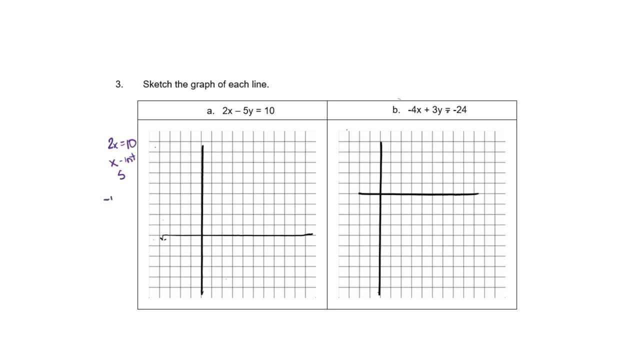 where x equals zero. so you can think about that in terms of the equation: negative 5y equals 10, which means the y-intercept is going to be negative 2.. I'm going to find those points on this graph: 1,, 2,, 3,, 4, 5, the x-intercept of 5 is going to go right there and negative 1,. 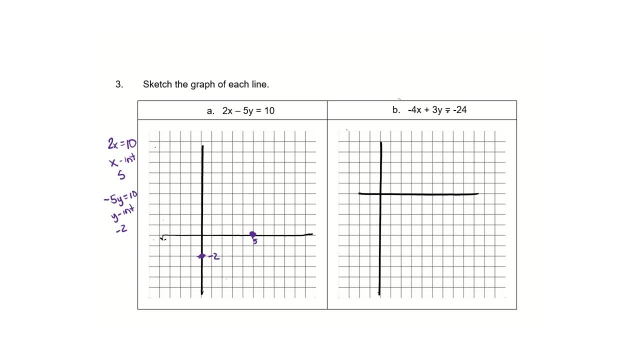 negative 2, the y-intercept of negative 2 is going to go right there, and so that's up two over five, 2 over 5.. That tells me that this is where my line is going to fall right here. So I will quickly. 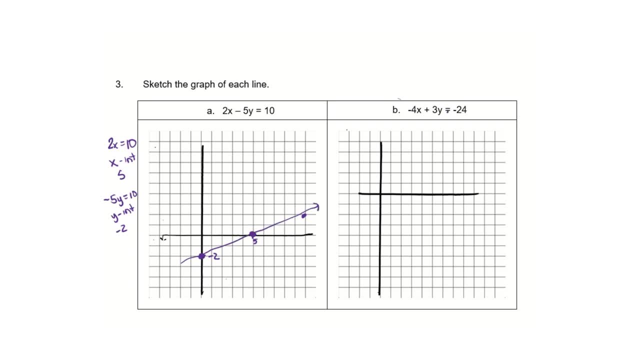 sketch the graph of that line and we will move on to the next example. So negative 4x plus 3y equals negative 24.. Again, to find the x-intercept, it's when y equals 0. So you're thinking about the. 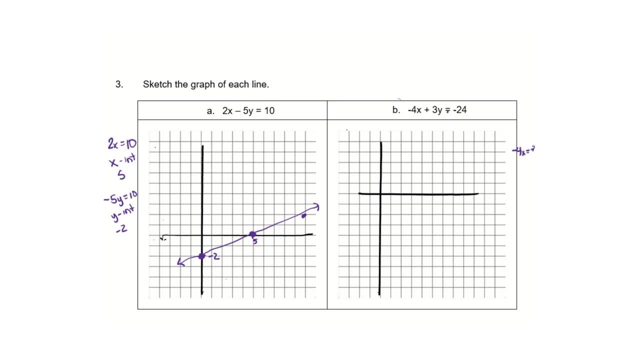 equation negative 4x equals negative 24.. So the x-intercept is going to be at positive 6.. And for the y-intercept you're thinking about, the equation 3y equals negative 24. So the y-intercept is going to be at negative 8.. So on the x-axis I need to find positive 6.. 1,, 2,, 3,, 4,, 5, 6.. 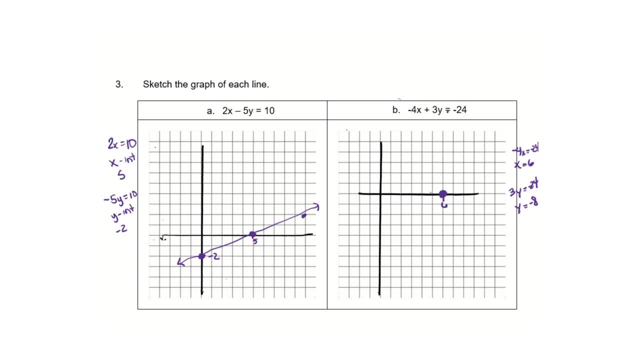 That's my x-intercept And my y-intercept. I need to find positive 6.. 1,, 2,, 3,, 4,, 5, 6.. That's my x-intercept And my y-intercept. 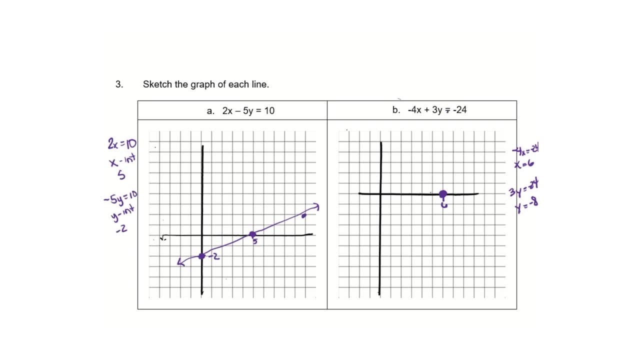 I need to find positive 6.. 1,, 2,, 3,, 4,, 5,, 6.. That's my x-intercept And my y-intercept. need to find negative eight. One, two, three, four, five, six, seven, eight. Negative eight. 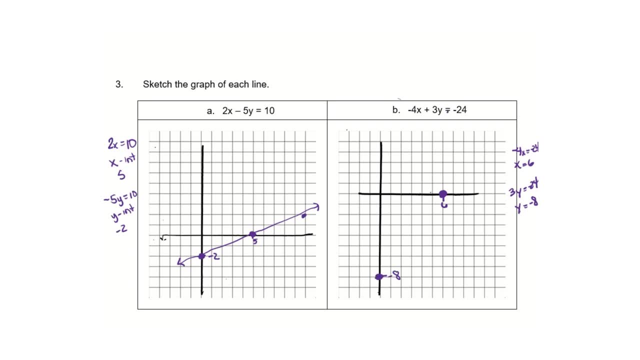 is where my y-intercept goes, and I'm going to go ahead and draw the line that connects those two points as my quick sketch. Fairly straightforward and simple once again, but you just need to understand the difference between when you use the x-intercept and y-intercept, or when you use 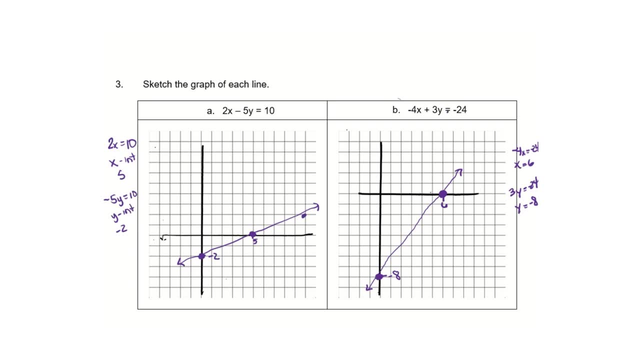 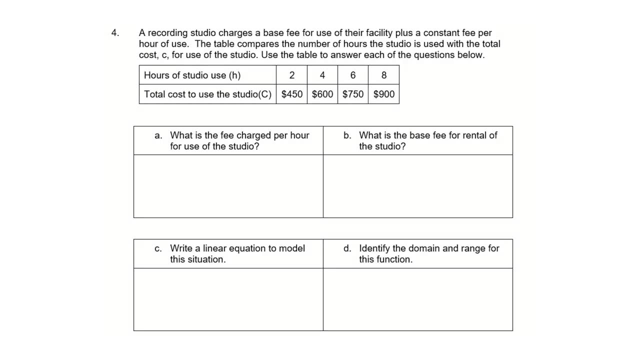 the y-intercept and then use the slope to find additional points. In problem number four we're going to get to application of these linear equations or linear functions. So number four says a recording studio charges a base fee for use of their facility plus a constant fee per hour. 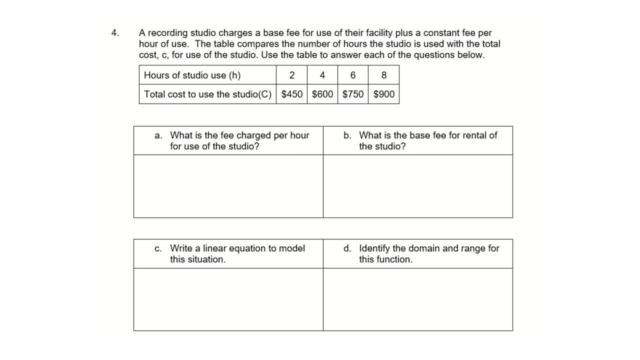 of use. The table compares the number of hours the studio is used with the total cost c for use of their facility. The table compares the number of hours the studio is used with the total cost c for use of the studio. Use the table to answer each of the questions below, And so you. 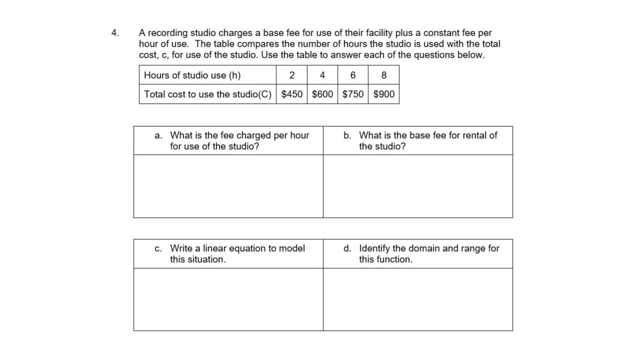 can see that two hours of studio use will result in a total cost of $450.. Four hours of use will result in a cost of $600.. For six hours it will cost $750, and for eight hours it will cost $900. 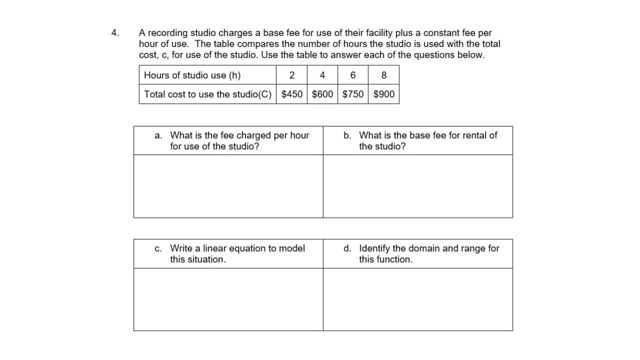 For part A, we're asked: what is the fee charged per hour for use of the studio? And if I'm just thinking about the situation and the cost of the studio, I'm going to go ahead and write down the cost of the studio And if I'm just thinking about the situation and I'm looking at that table, 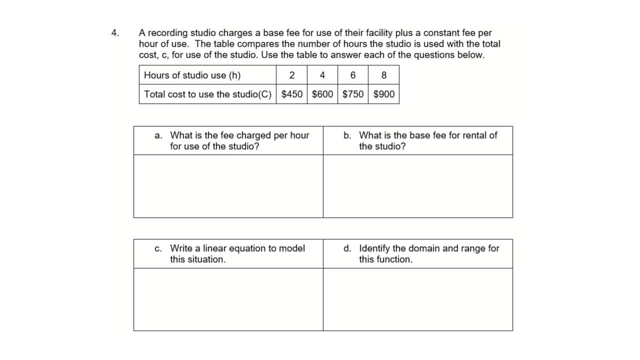 one of the things that I would notice is that when we increase by two hours, we're increasing by a total of $150.. So for two hours of use it's going to be $150.. That would mean that for one hour of use the cost is $75, right? If we wanted to formally calculate this, we could essentially. 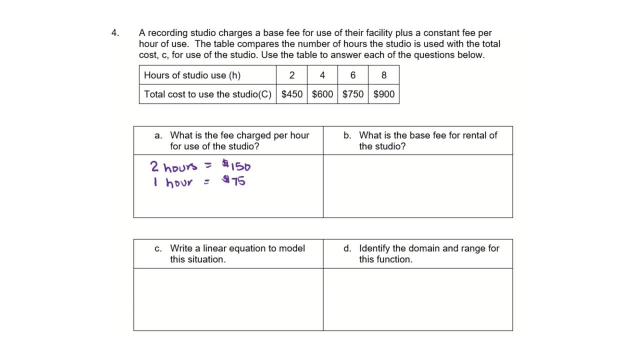 find the slope. But if we wanted to formally calculate this, we could essentially find the slope. But if we wanted to formally calculate this, we could essentially find the slope, But between two points. So for example, if we use the two hours, $450 and the four hours, $600,. 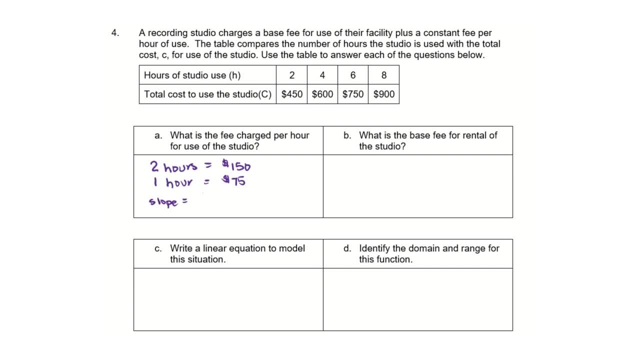 the slope of this line would be $600 minus $450, because that's the y-coordinates- over four hours minus two hours because those are the x-coordinates. So that's $150 over two or $75 dollars per hour For part B. what is the base fee for rental of the studio? 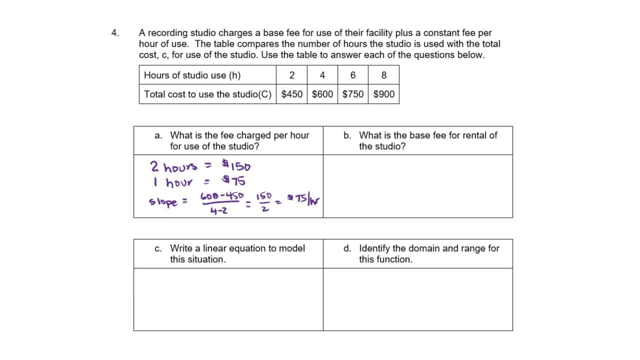 That's like what is the amount that we have to pay in addition to the hourly rate right? So if two hours costs a total of $450, and we know that two hours the hourly rate времени is $150 overall – two hours at the hourly rate will cost me $150. 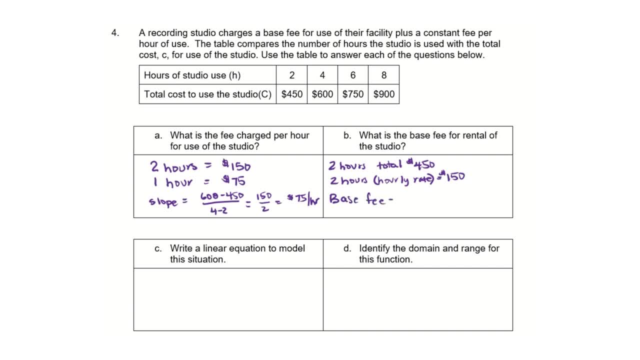 Then that has to mean that the base fee $300. And we would get that because that's the difference between the total cost at the hourly rate. Now I can write my linear equation. My linear equation is going to be: my total cost is equal to $75 for each hour that I 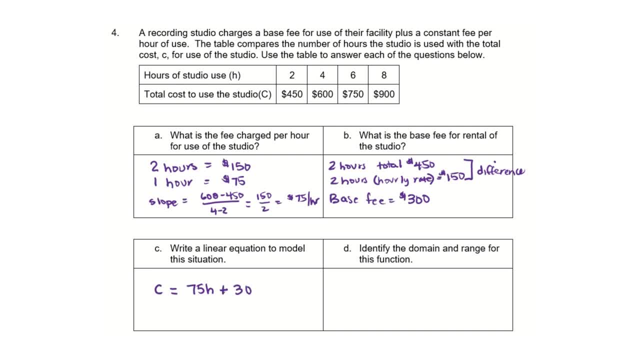 use the studio plus that $300 base fee, And when I think about the domain and range in Part D, the domain hours would have to be greater than zero. right, I'm not going to rent the studio and then not use it. 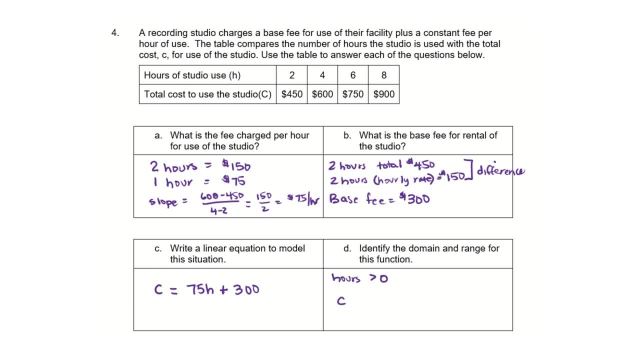 So my hours have to be greater than zero And my cost then has to be greater than $300 because, again, I'm not going to rent the studio and not use it, which means I'm going to pay that $300, plus, I'm going to pay something. 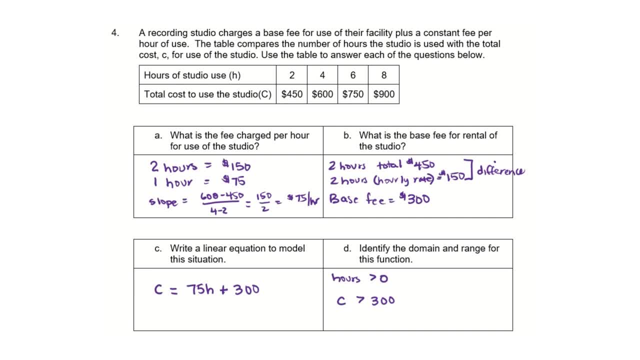 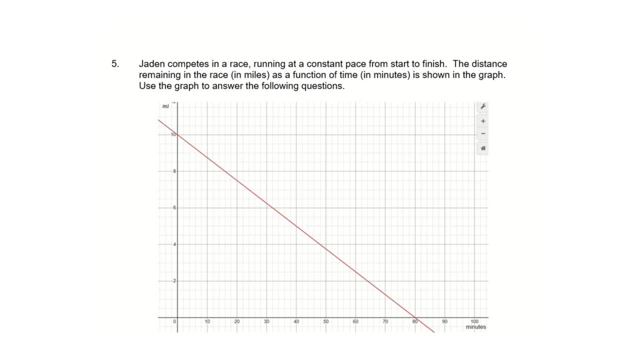 else on top of that for an hourly rate. So it would be greater than $300.. Problem number five is another application problem. Jaden competes in a race Running at a constant pace from start to finish. The distance remaining in the race in miles as a function of time in minutes, is shown. 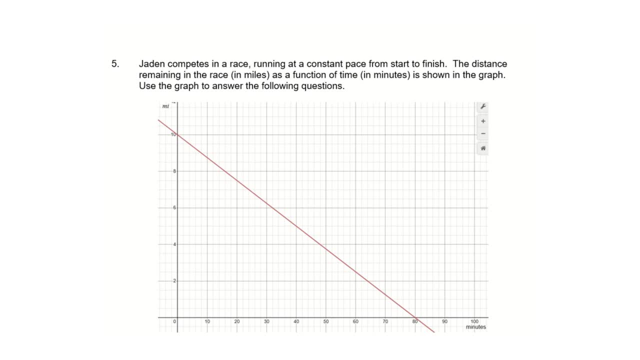 in the graph. Use the graph to answer the following questions. Well, before we even dive into the questions, let's take a close look at the graph and see what we have. We've got a line that crosses the y-axis at 10, right. 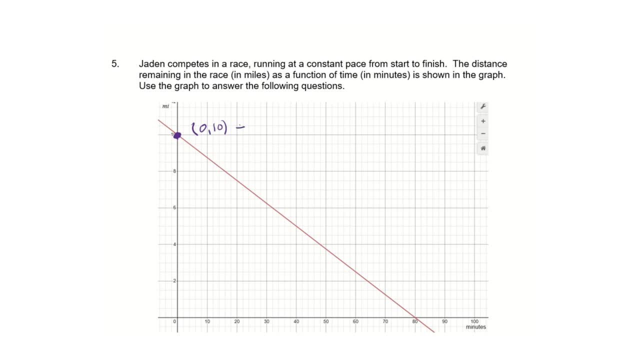 So the coordinates of that line are 0, 10.. And the meaning of that is zero minutes. So let's go ahead and place the figure here to the new question. So 10 minutes have passed And 10 miles remain in the race. 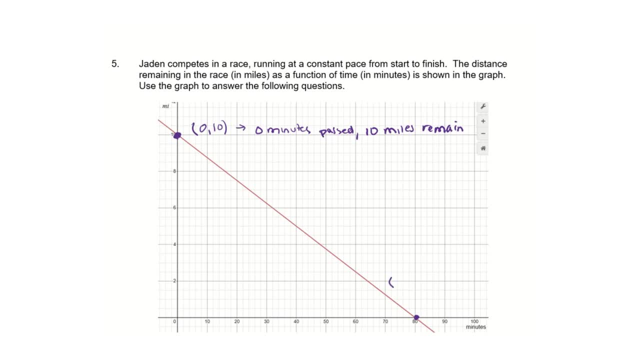 The other important point on this graph is where it crosses the x-axis, And the coordinates of that point are 80 and zero, And the meaning of that point is: 80 minutes have passed. Do you think too? We are thinking- and 0 miles remain, The other thing that we should probably think about, since we 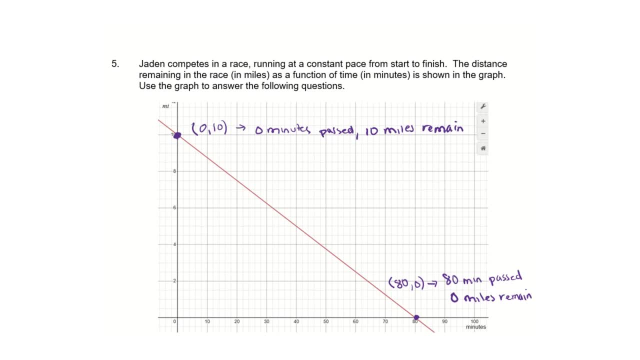 always get asked about it when we're looking at examples of lines: is the slope of this line? If I think about the slope of this line, we now have the coordinates of two of the points on the line, so we should be able to calculate. 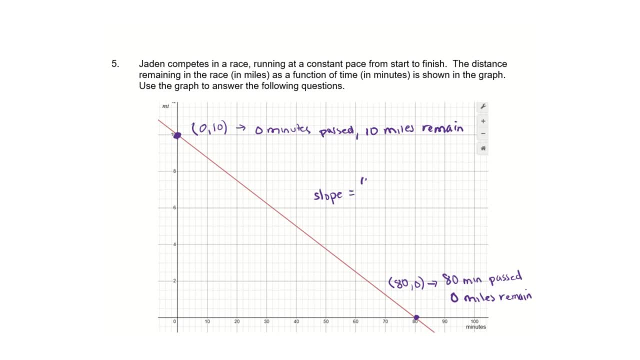 the slope. We subtract the y-coordinates, so 10 minus 0, and we subtract the x-coordinates in the same order that we subtracted the y-coordinates, so 0 minus 80. And when we simplify this, we have 10 over negative 80,, which is the same thing. 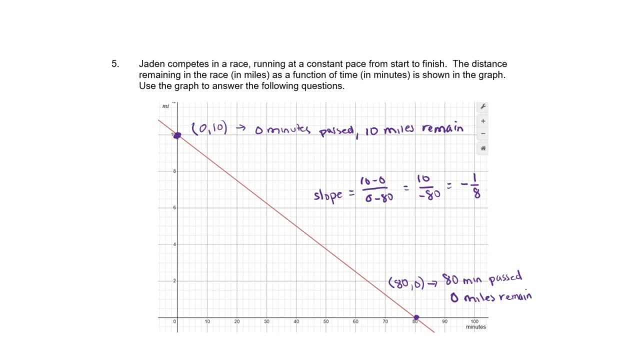 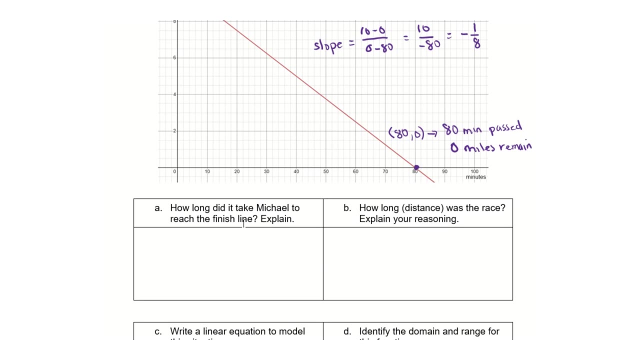 as negative 1- 8th. So we've dissected a lot of information before we've even looked at what our questions are. Let's go look at our questions now. So part A says how long did it take Michael to reach the finish line? And 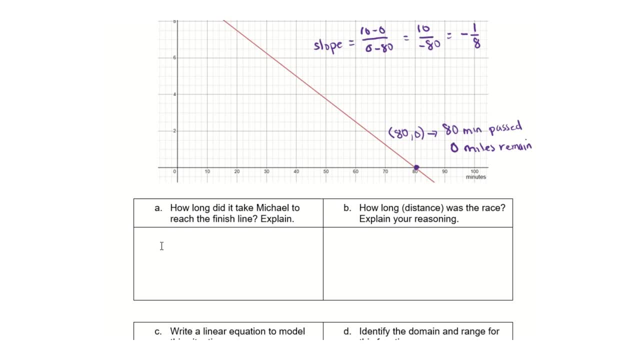 explain our answer. Well, if I look at where he's at when 0 miles remain, we saw that it took him 80 minutes to get to the point where 0 miles remain. So the 80 minutes represents the x-intercept or the point. 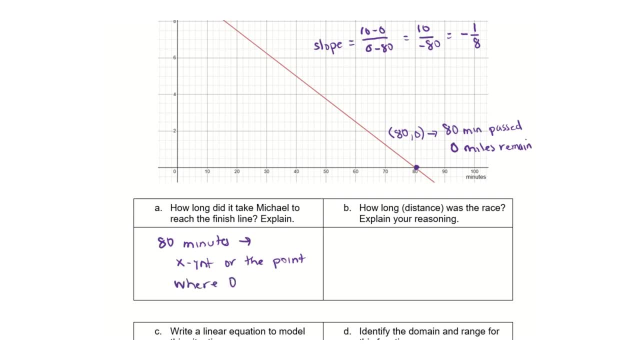 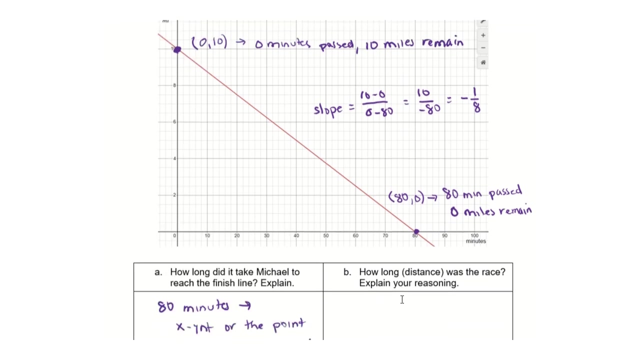 where 0 miles remain. Part B asks how long was the race And explain our reasoning. And if we go back to the y-intercept, what we'll see on the y-intercept is, when 0 minutes have passed, 10 miles remain. So that's his starting point. No time has gone by, but 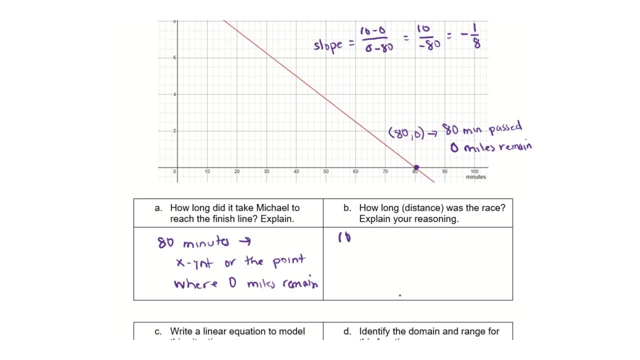 he's at 10 miles. So the answer to the question is 10 miles and we know that because it's the y-intercept And that's the point where no time has passed For part C. we're asked to write a linear equation to model this situation. If we're 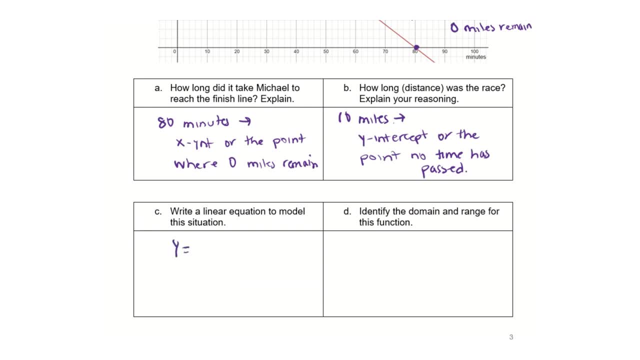 going to write a linear equation to model this situation. we're going to have to write a linear equation to model this situation. If we're going to write a linear equation to model this situation, we have everything we need to write this equation in slope-intercept. 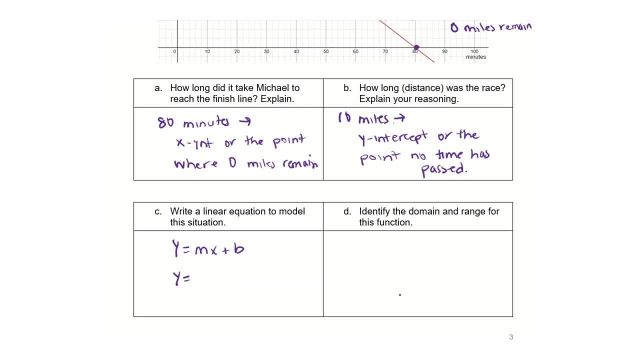 form, which is: y equals mx plus b. We know that the slope is negative 1 eighth, and we know that the y-intercept is 10.. So our equation is: y equals negative 1 eighth, x plus 10.. And then, when we identify the domain and range for this function, it's going to be important. 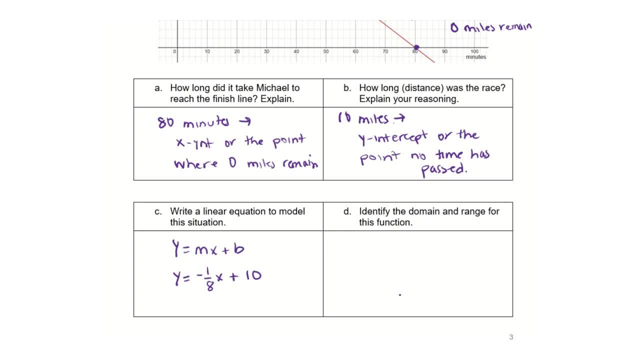 to note that we can't consider negative minutes. and we can't consider negative minutes, So we're going to have to write this equation in slope-intercept form, which is: y equals 0 minus 10.. So we're going to have to write this equation in slope-intercept form, which: